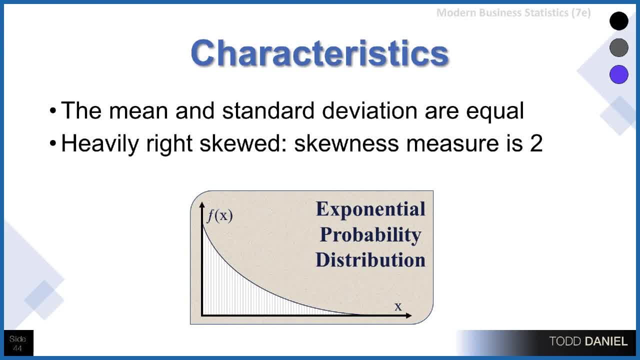 of this exponential distribution, The mean and the standard deviation- and this is also like a Poisson distribution- are equal, But the exponential probability distribution is heavily right side. So the mean and the standard deviation- and this is also like a Poisson distribution. 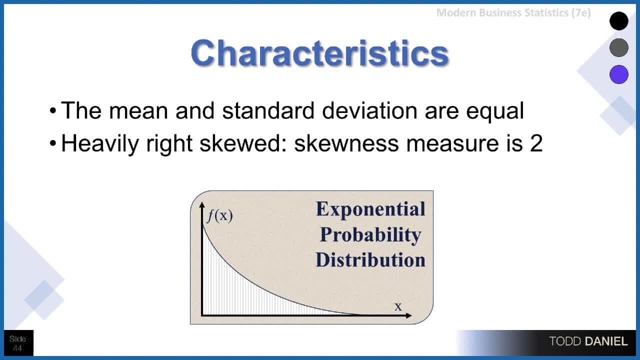 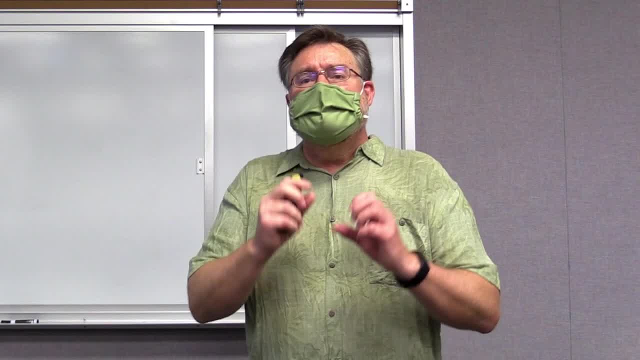 are skewed. In fact, if we look at the skewness measure, it will be equal to the number two, And I promised I would clarify between an exponential and a Poisson distribution. Poisson in the Poisson distribution the word in French means fish, So I thought maybe a fishing analogy. 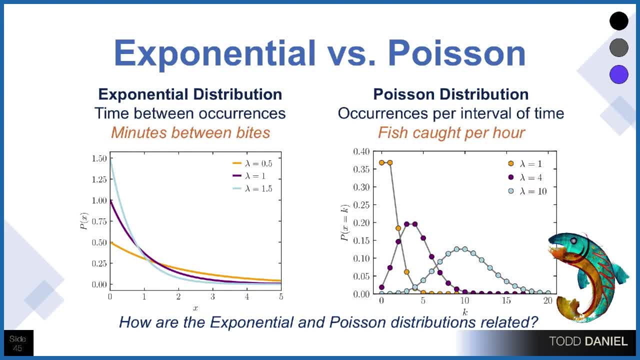 would help. A Poisson distribution is the occurrences per interval of time. So if we're spending spring break on the lake doing some fishing, the number of fish caught during the break would be equal to the number of fish caught during the break. So the number of fish 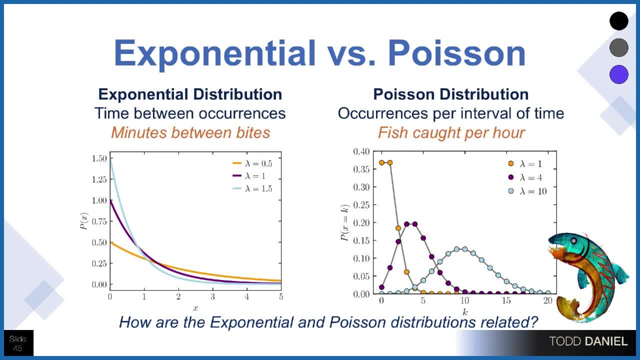 caught per hour would be, would follow a Poisson distribution: occurrences per interval of time, But the exponential distribution is the time between occurrences, the number of minutes that elapse between bites, between strikes on the line of a fish that may potentially end up in the boat. 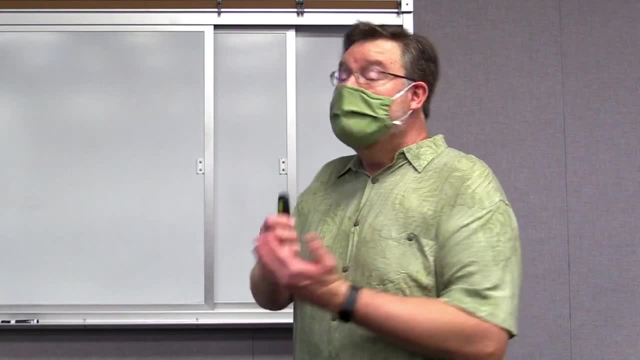 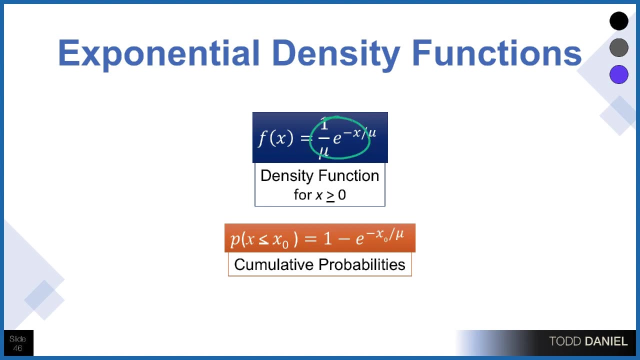 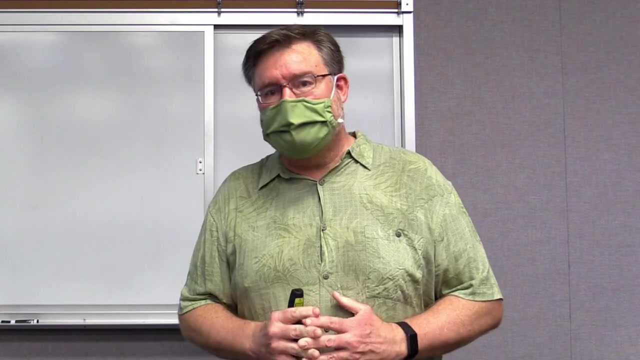 And this gives us an idea of how the exponential distribution is calculated. Here is the probability density function. You'll notice that letter E, Euler's number, And you will see the cumulative probabilities also with that letter E. And, as before, you did not need to memorize these distributions or these formulas. but here, 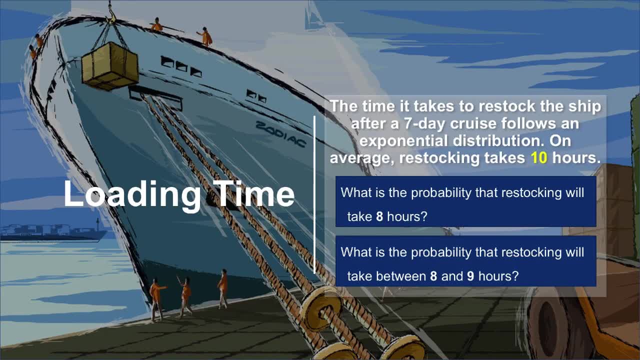 is how we could use them in the real world. The time it takes to restock the ship after a seven-day cruise follows an exponential distribution. On average, the number of fish Τc- The existence and efficiency of the Hi- coal reactor- excites about 600 people daily. 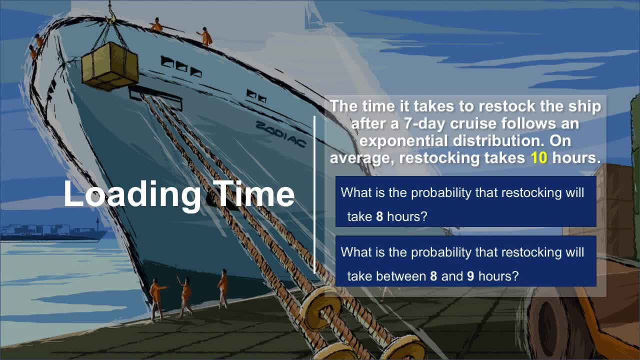 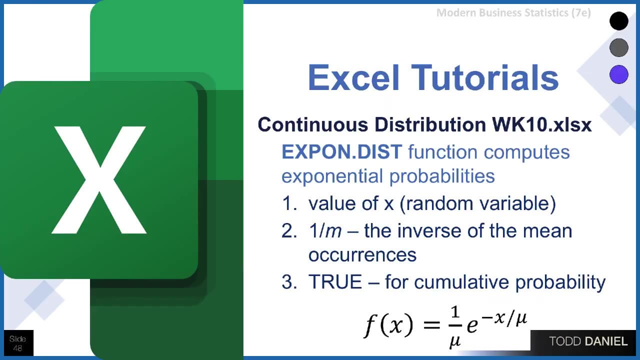 Restocking takes 10 hours, What is the probability that deed会 8 часов? What is the probability that restocking will take between 8 and 9 hours? To answer these questions, I have another spreadsheet that I would encourage you to use. 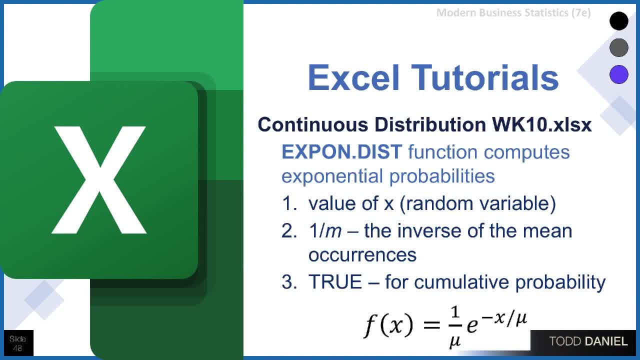 This is the Continuous Distribution Week 10 Excel Spreadsheet. This is where I use the exponential distribution function to answer these questions. You'll see in the upper-left corner, below the expression and gram level of fresh water. The expression is multiplied by the amount of liquid to be Day byphy, by the amount of LISA of starch. 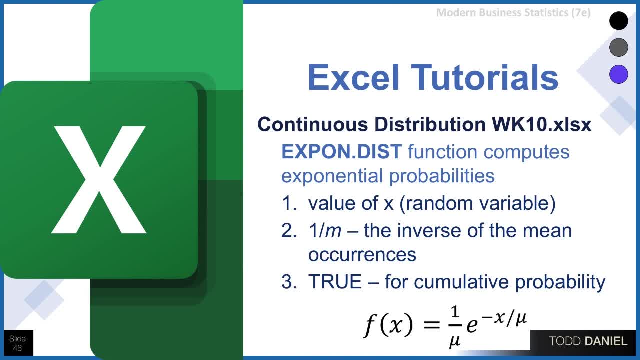 within a 어� hemimic recycle bubble. I've recorded the moment of conservance as shown along right side, right now very significant waterpor Ll. But this is by continuation. What you will need, or subtract, is three. The exponential distribution function has three arguments. 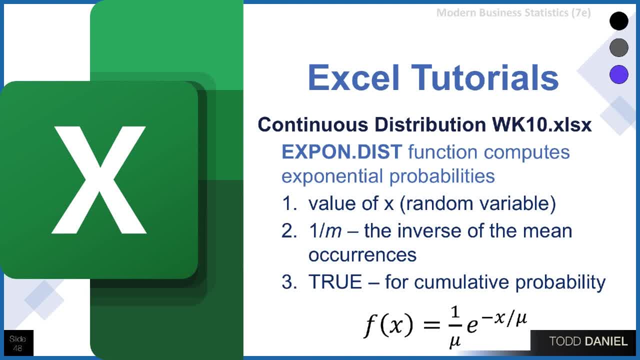 The first is the value of X, the random variable. The second is the inverse of the mean, or one over M, one divided by M, And the third is true, which gives us a cumulative probability. That's what we will use for all of these examples. 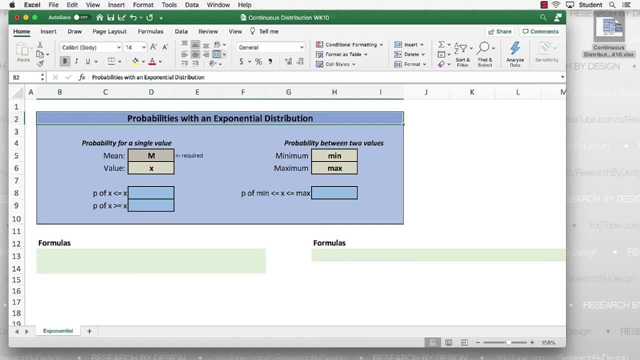 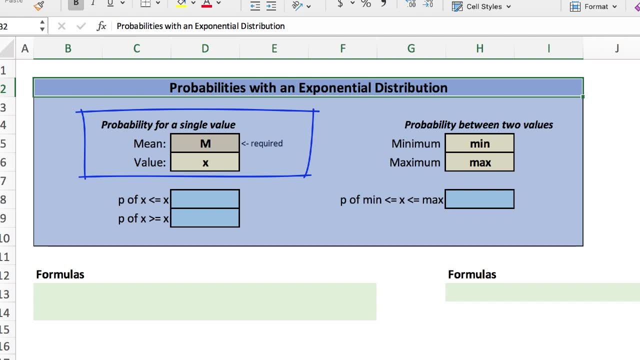 If you open up the continuous distribution, week 10 Excel spreadsheet, you'll see it looks like this and we'll need to enter the mean and some values in order to get the probabilities. The first thing we'll enter is a mean of 10.. 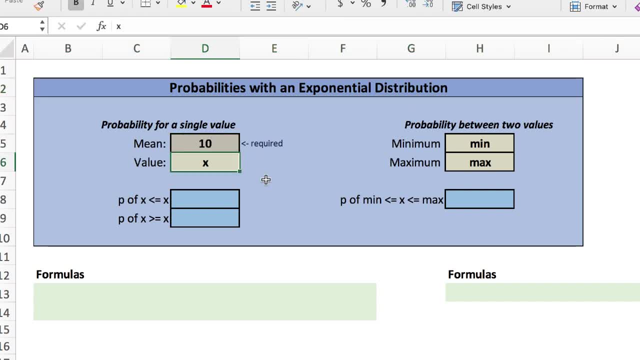 Now that is required to use this spreadsheet And we want to know the probability of the load time taking eight hours. We'll put that value right below the mean. it's a value of eight and we get the probability as a 0.5507. 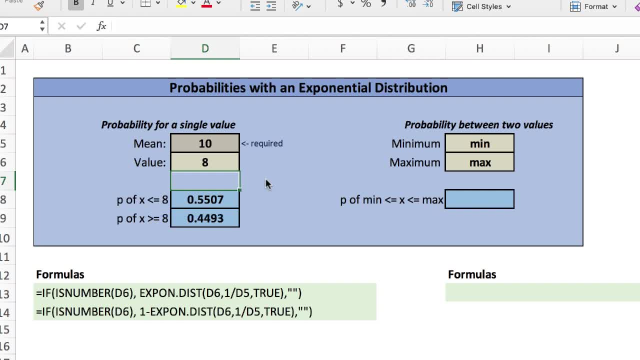 That's a probability. That's a probability. That's a probability less than eight. and I've also added four of the probabilities greater than. If we want scores between two given values, we would enter those as the minimum and the maximum. let's say eight and nine. 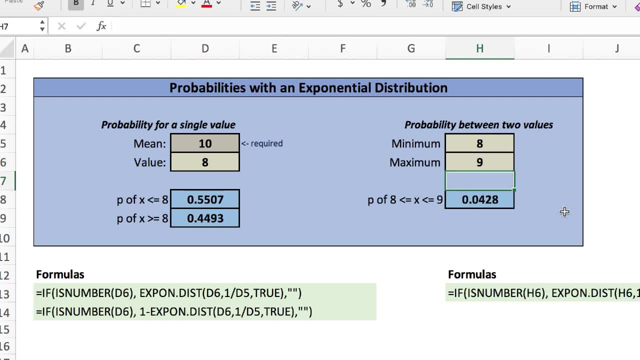 And this gives me the probability between those two. So roughly 4% of the time would we have a load time between eight and nine hours. As you fill in these numbers, you will notice things change throughout the spreadsheet, including you will be able to see the formulas that you've entered for each of these examples. 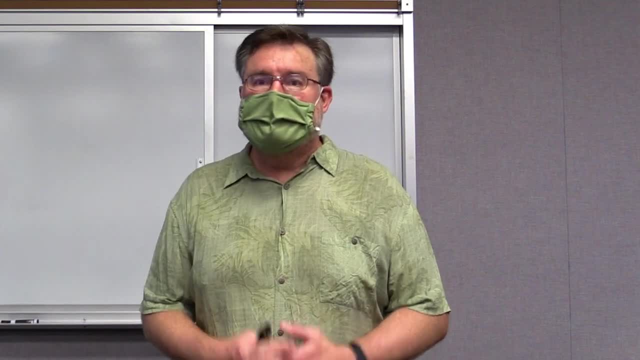 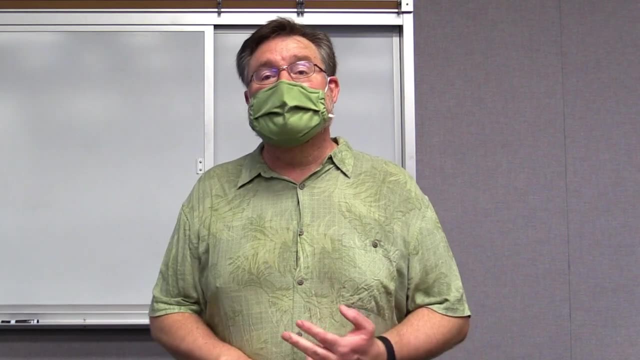 And that's what we need to cover for exponential distributions. All right, those are our three distributions. We have the uniform distribution, the normal distribution, which we'll use a lot, and the exponential distribution. So do you have any questions? before we wrap up today, 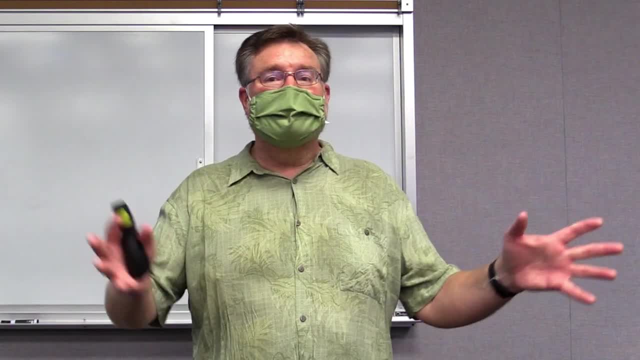 I want to say thank you to all of you for being here. Hope you have a great spring break. Thanks everyone, I'll see you next time. Bye-bye, Bye-bye.